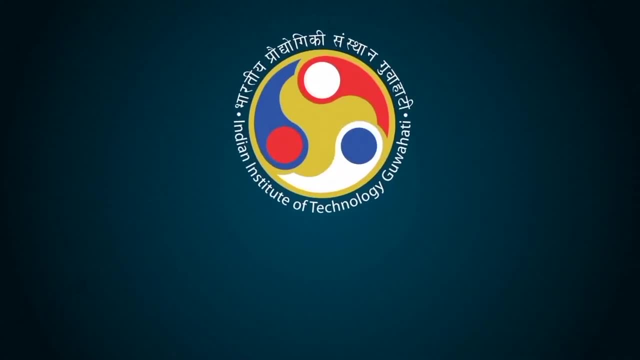 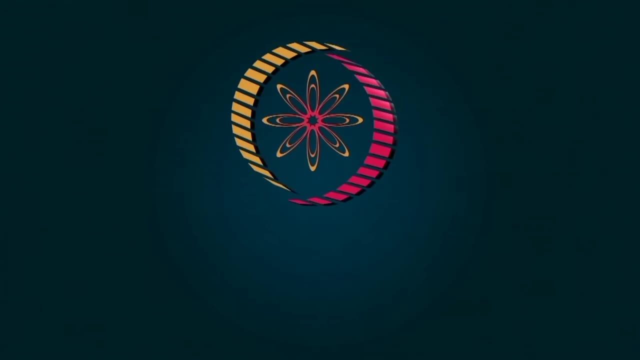 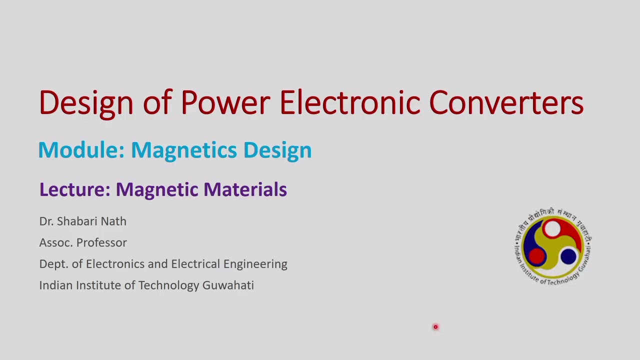 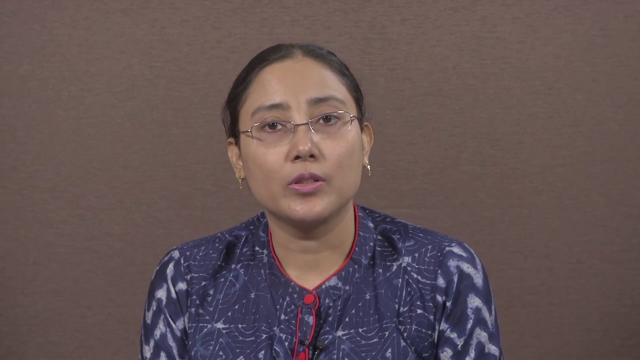 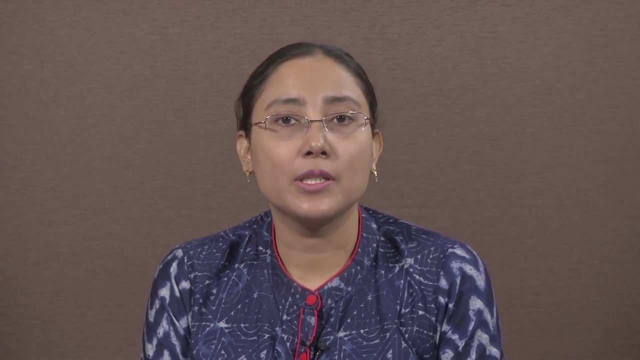 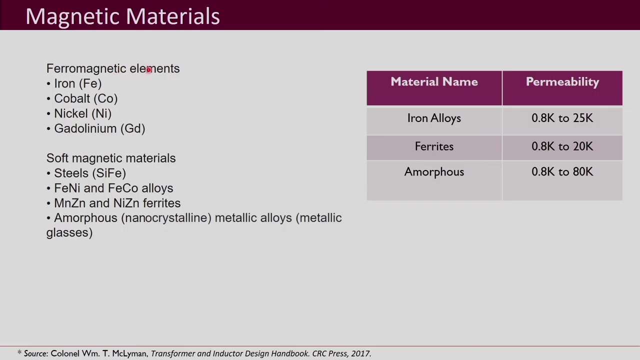 Welcome to the course on design of power electronic converters. We were discussing magnetics design, So let us now look into the different magnetic materials that are used for making your magnetic cores. So the materials which are used for making magnetic cores are basically your ferromagnetic. 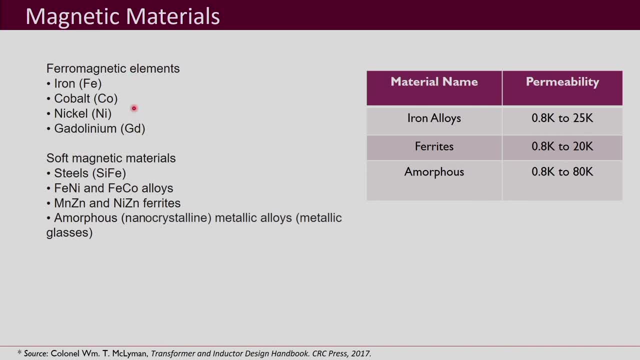 elements, and these are the main ferromagnetic elements: iron, cobalt, nickel and gadolina, And there combinations are many times used to make what are called as the soft magnetic materials. So soft magnetic materials mainly are of 4 types: your steel based and second is your 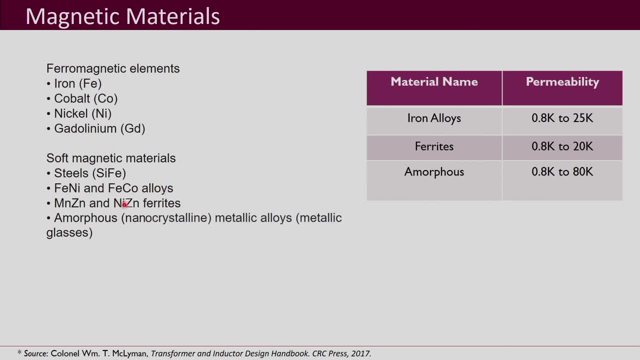 iron alloys. Apart from that there are ferrites and then there is amorphous material which can be of metallic glass. So your permeability range is shown here for iron alloys. this is the permeability range, and then for ferrites and amorphous, it is shown here, So you can see that amorphous. 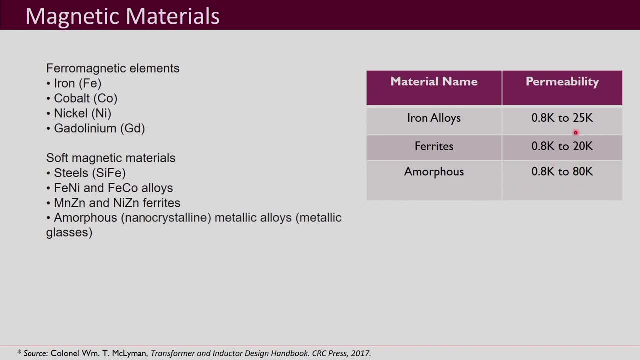 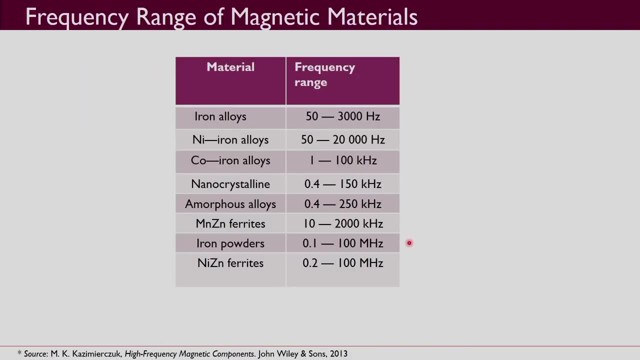 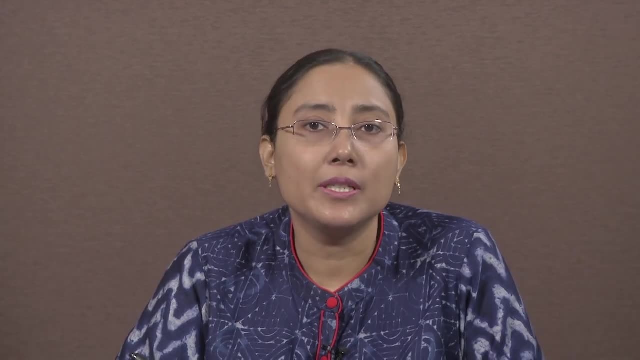 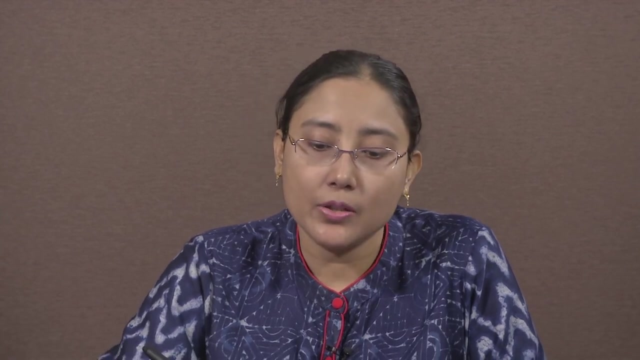 materials have relatively much higher permeability range as compared to your iron alloys and ferrites. So if you select a magnetic material for a particular power electronic application, then we have to see whether the material that we are choosing, whether it is suitable for the frequency of operation or not. Now this table shows the frequency range of magnetic. 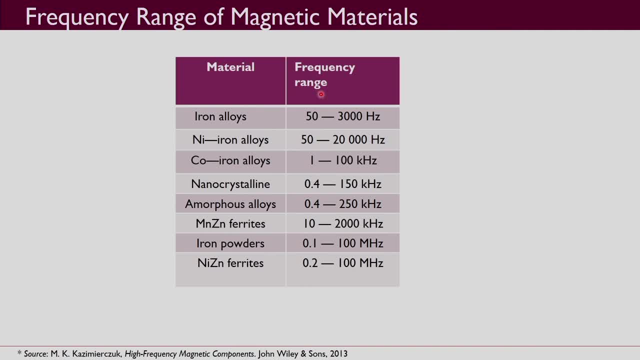 materials. You can see here that iron alloys are. their frequency range is relatively lesser. So 50 to 3000 hertz, that means 3 kilohertz, is the frequency range in which your iron alloys can be used, For example your CRGO cold rule gain oriented steel you might have. 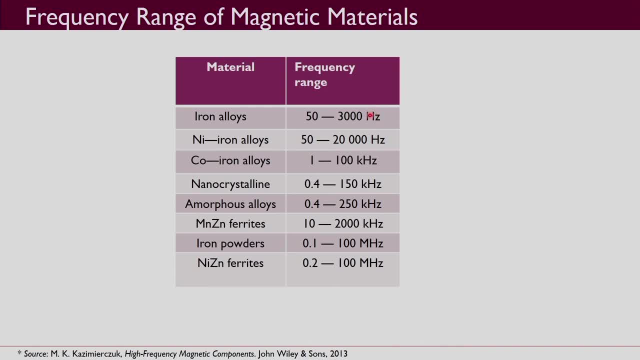 heard about. it is what is used in your 50 hertz power transformers And then your other, which is nickel iron alloys or cobalt iron alloys. their frequency range is Relatively higher. Further as you go to nano crystalline and amorphous alloys, their frequency 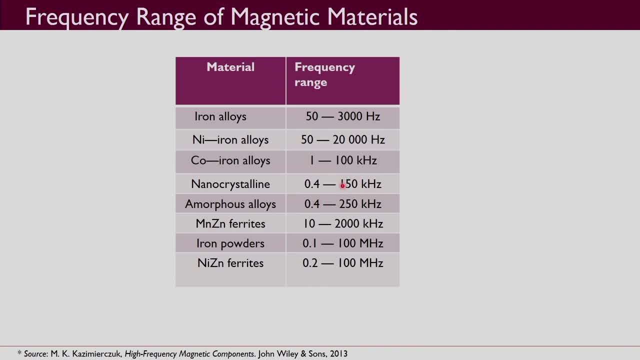 range is also good. It is up. nano crystalline materials can be used up to 150 kilohertz and amorphous alloys can be used to about 250 kilohertz. Then comes your ferrites. ferrites, the frequency range, your manganese zinc ferrites. their frequency range is also good, uptes out. 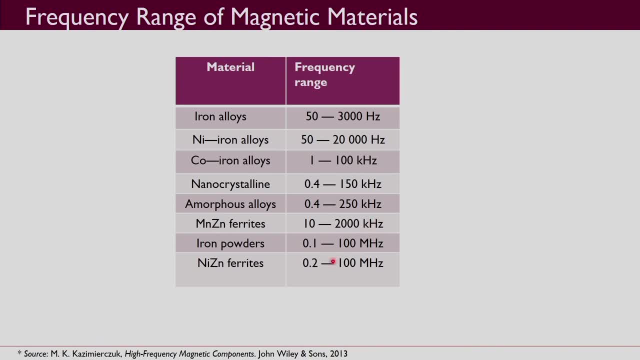 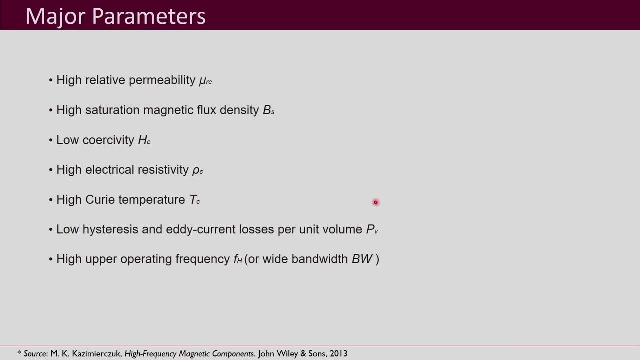 about 2 megahertz. they can be used The iron powders and your nickel, zinc based ferrites. their frequency range is even higher. they can be used up to about 100 megahertz. So the important parameters that that you should be looking into when you select a magnetic. 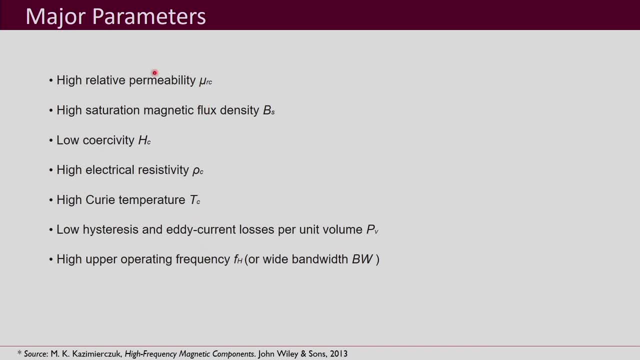 material. those are given here. one is your. this high relative permeability. the relative permeability of the material should be very high, as high as possible. Then the saturation flux density. it is desirable to have high saturation flux density, then low coercivity, hc, because coercivity is something, is what is required, the coercive force to 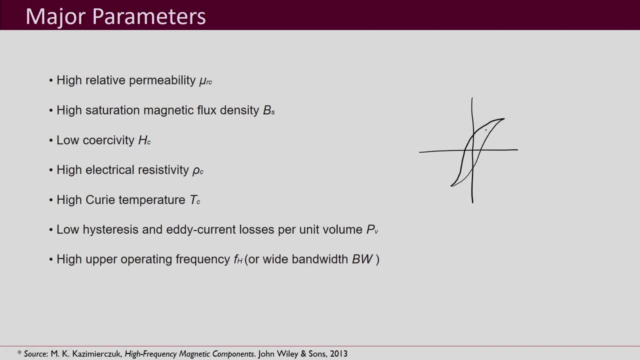 make the magnetic field flux density equal to 0. So this gives your hc. So this is your bh curve. So this part is your coercivity and this part is your residual flux, can call it as the br. So this should be as low as possible, the hc value. 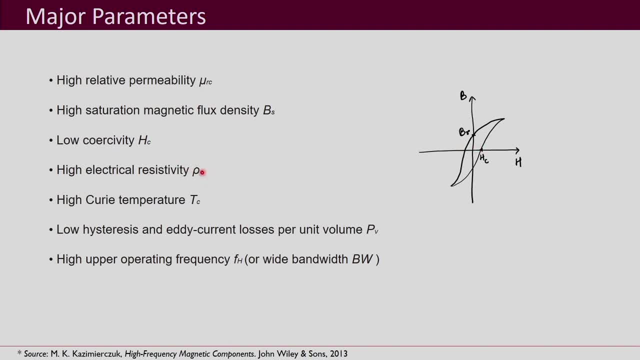 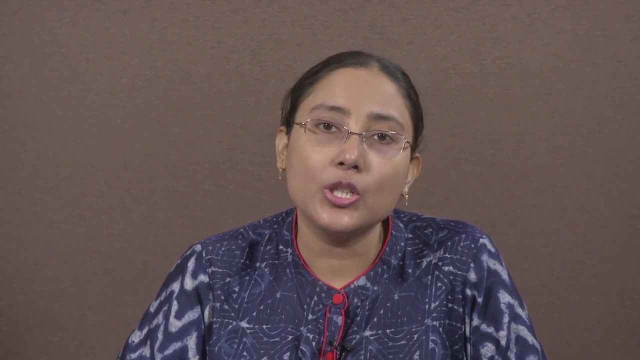 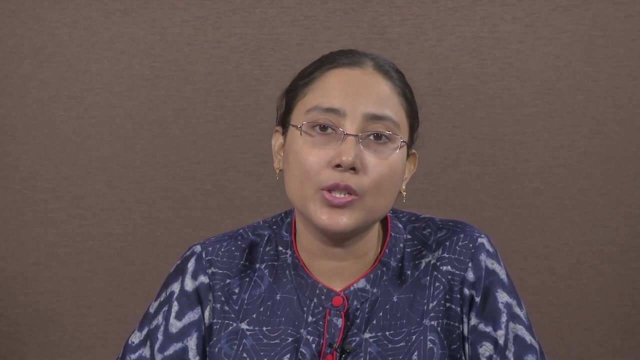 Then high electrical resistivity, rho c. Now why electrical resistivity is important. this we have discussed before about eddy currents. So whenever we choose a magnetic core, then there will be eddy currents in it and they should be as less as possible. So one of the ways of reducing eddy currents by laminations, but not all materials may support. 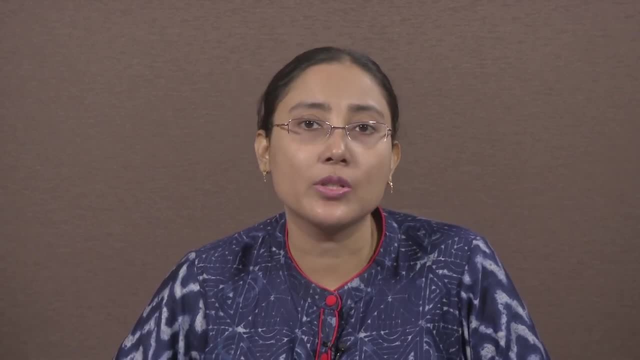 formation of laminations. because they will be brittle material, laminations cannot be formed. Apart from that, we order the stacking of the laminations. So for now I am done with my presentation. I hope that you have found it helpful. Don't forget to subscribe. 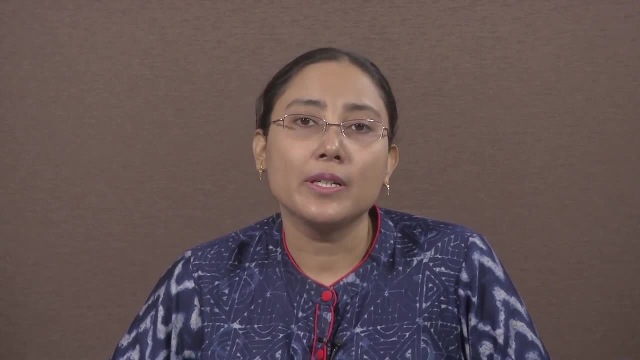 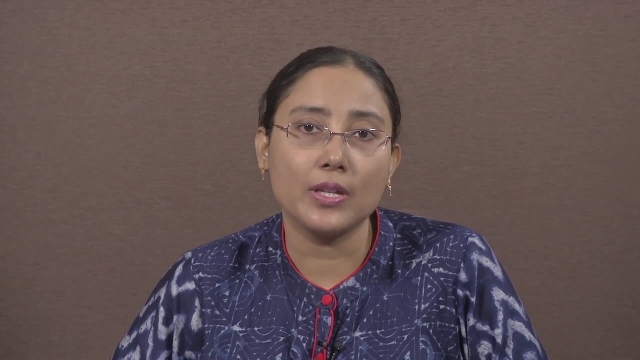 See you in the future. Bye, Bye, Bye, Bye, Bye is also a problem. So it is better to have a solid course, but then for that your resistivity of the material should be high, So that the eddy currents that are produced would be less. 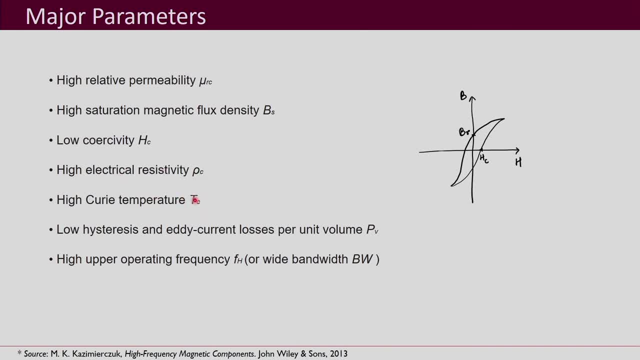 Then high Curie temperature. Now, what is this Curie temperature? It is the temperature at which the magnetism is lost. This is a very rough definition. There are more precise definition, but for our purpose, for simplicity, just understand that Curie temperature should be very high. 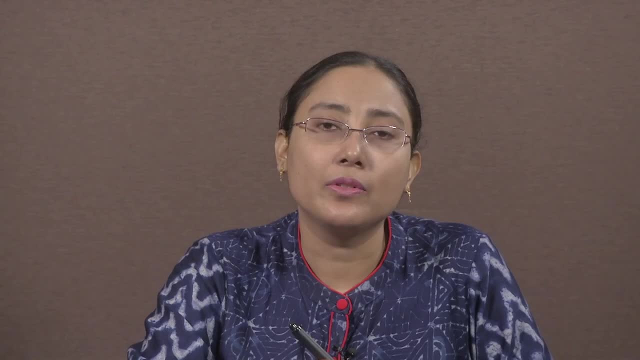 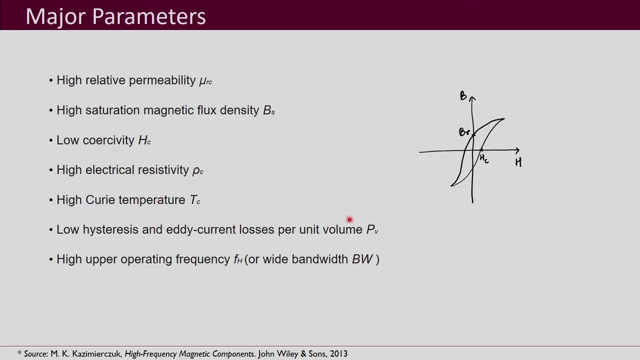 The higher it is, the more is the ability of the material to withstand your temperature. A low, hysteresis and eddy current losses per unit volume PV. So the loss that is going to take place, the core loss, that should be low and per unit volume loss, this parameter. 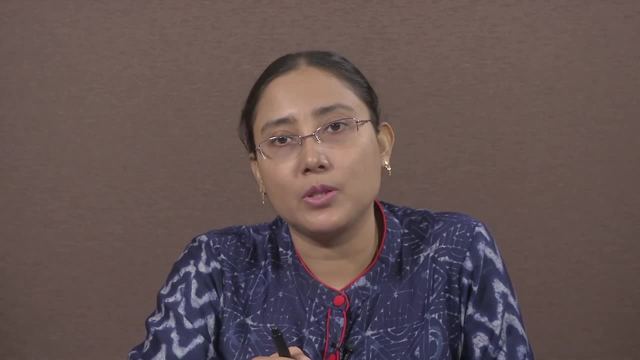 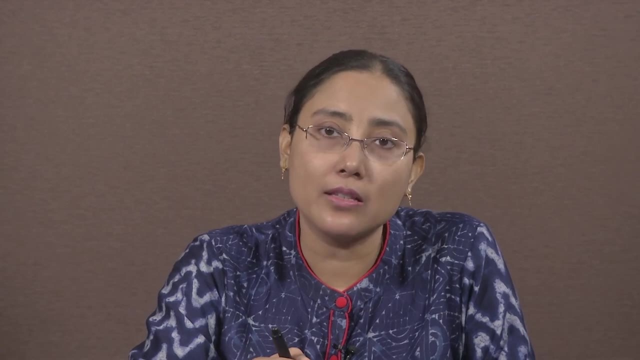 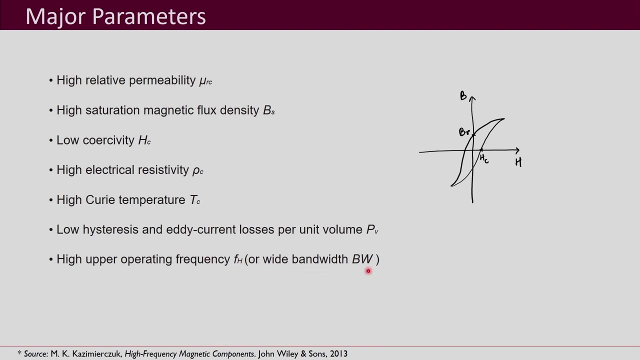 is provided by the Manufacturer of these magnetic materials, and so you should look into it that this PV value, the core loss value per unit volume, should be as low as possible. Then your high upper operating frequency range. So if you have very high frequency range up. 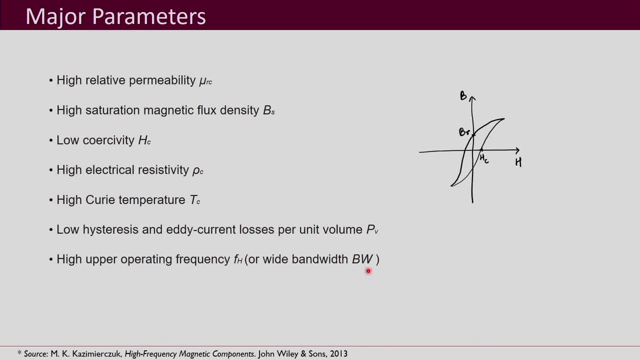 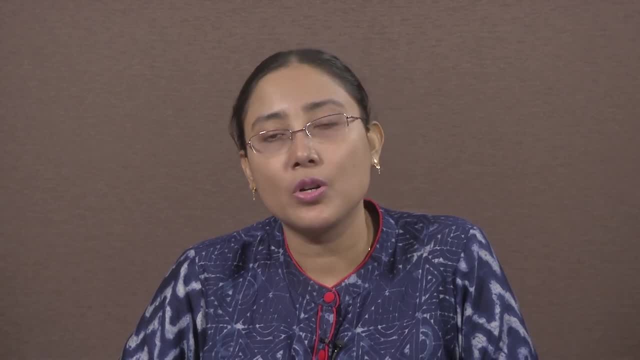 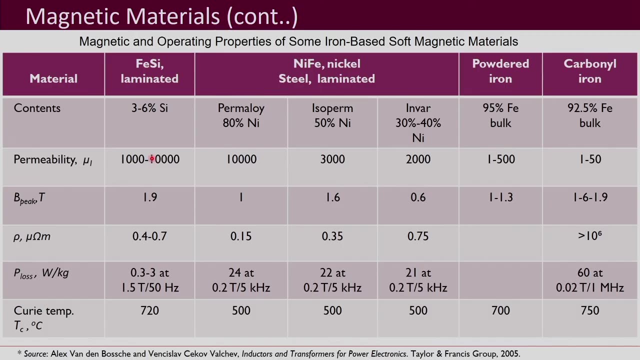 to which this the material can be used. so then that is very good. you can use it for wider frequency ranges. But, however, depending on your particular requirement of frequency, you should be looking into Whether the material can be used for those ranges of frequencies or not. This is a table. 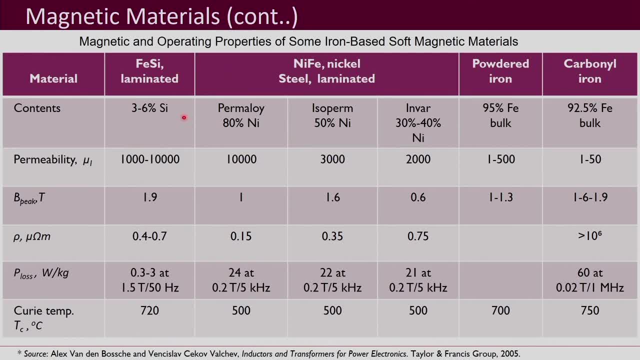 which shows the properties of these iron based soft magnetic materials, mainly your iron silicon, then nickel iron and powdered iron and carbonyl iron, And but they have their own composition here. This is 6 percent of silicon, and this nickel iron again can be made in different compositions. 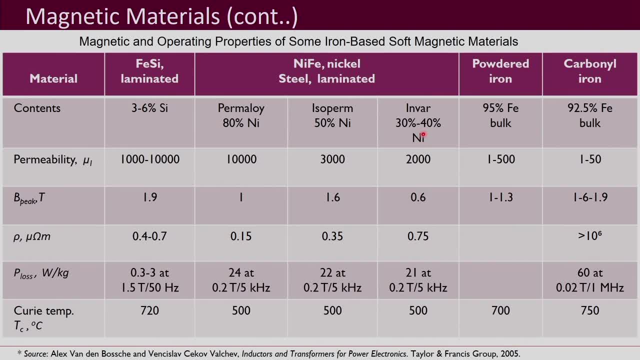 so that is given for three compositions over here in this table: Then powdered iron composition and then your carbonyl iron. So first is your permeability, which is very, very important. it should be as high as possible. So if you see here carbonyl irons, permeability is much. 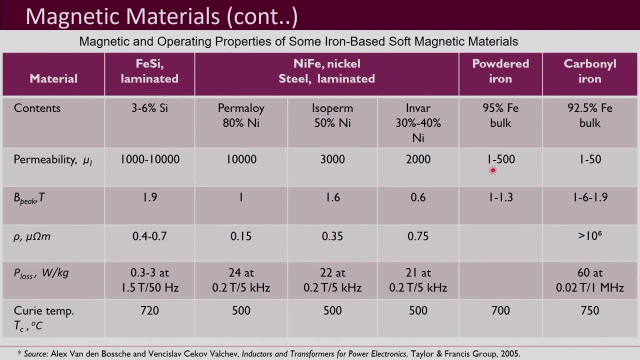 lesser And as we go to powdered iron it increases. then for nickel iron it is further high and it depends on the composition of pure of the material that is being used. And then further your iron silicon. this material has this very good permeability range of 1000 to 10000. 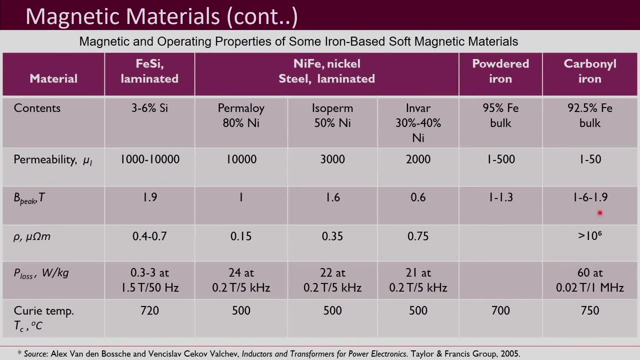 Then B peak, that means your saturation flux density. If you see here this is a very good permeability range of 1000 to 10000.. Then B peak, that means your saturation flux density. Then the highest that we see here is 1.9. and nickel: iron: for your isoperm, 50 percent nickel. 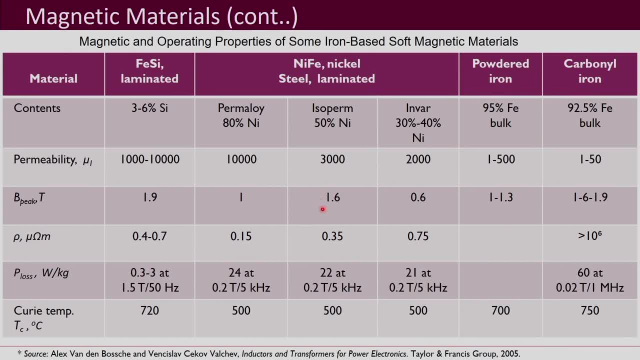 there also. you see, the saturation flux density is quite good, it is about 1.6, and carbonyl iron also has good saturation flux density. Then, further your resistivity, it should be as high as possible. Now here you see, all of these have lower resistivities, whereas this one, carbonyl iron- this has got. 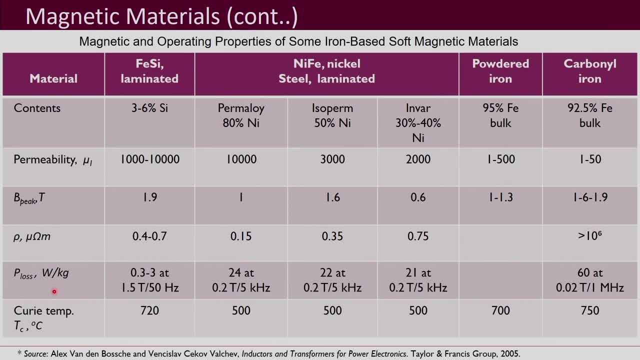 very good resistivity And p loss. this should be as low as possible and here, if you compare it, you can see here that this iron silicon is what which has very low p loss, And of course this is measured at a particular flux density. so 1.5 tesla. And for a particular flux density, it is 1.5 tesla. So 1.5 tesla is the same as 1.5 tesla. So 1.5 tesla is the same as 1.5 tesla. 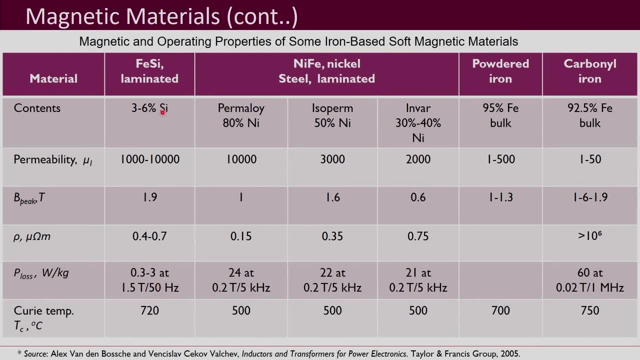 So 1.5 tesla will be your particular frequency, which is your 50 hertz, and this material is iron silicon, which is specially used for your 50 hertz power transformer applications. Then your curie temperature. curie temperature should be as high as possible. 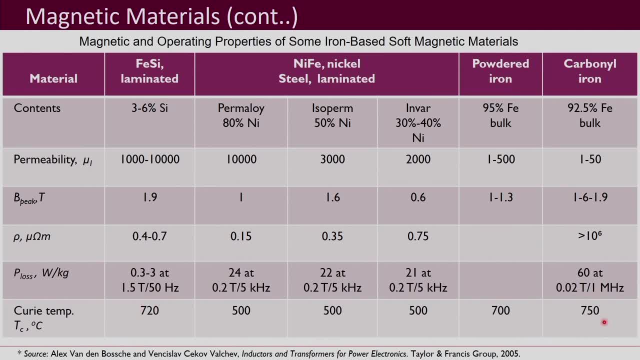 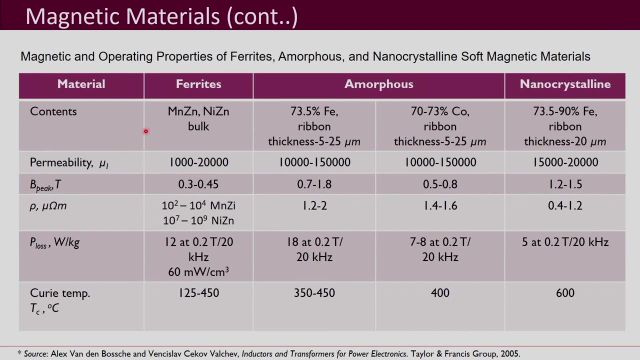 So here you can see that that iron silicon and your carbonyl iron, these two have got very good curie temperature and the powder iron also has a very high curie temperature. data is given here for ferrites, amorphous and nano crystalline material. 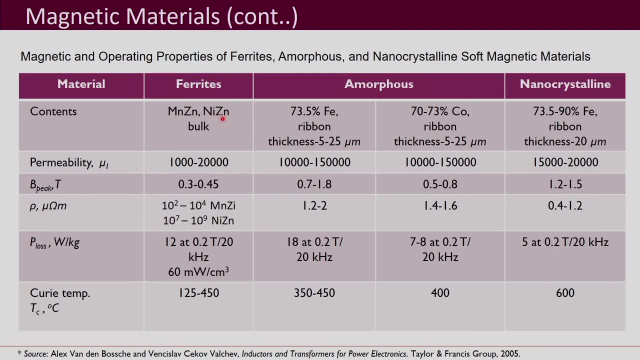 So ferrites your in. they come in different composition: manganese, zinc- different elements may be used here- And amorphous again. they can also be manufactured using different elements and different compositions. So this is what is given here for this composition: 73.5 percent iron. 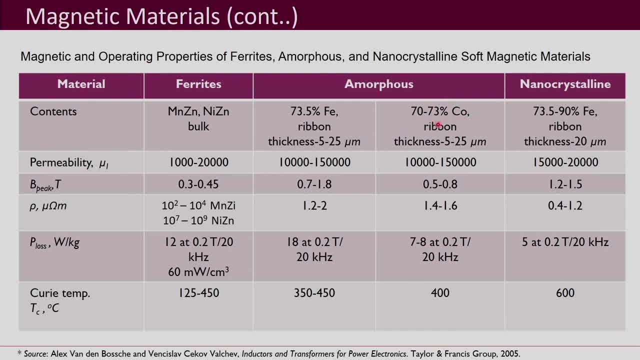 Then this one is for 72, 73 percent of cobalt and then nano crystalline material. the composition there here it is used, consist of 73.5 to 90 percent of iron. So permeability range. if you see, all of these have very good permeability okay. 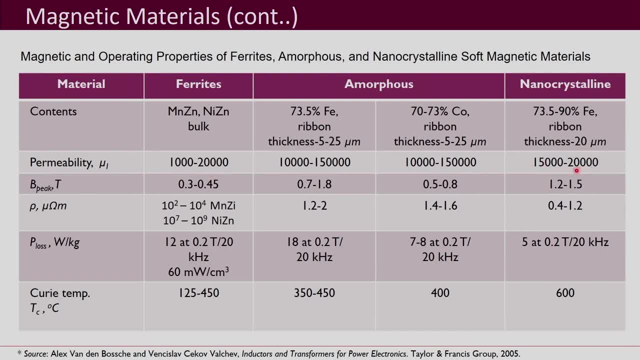 Your nano crystalline has very high permeability. Then saturation flux density. if you see saturation flux density, Okay, Of your ferrites is relatively less So, although it can be used for very high frequencies, but the problem is that that it you cannot push lot of flux density through it. 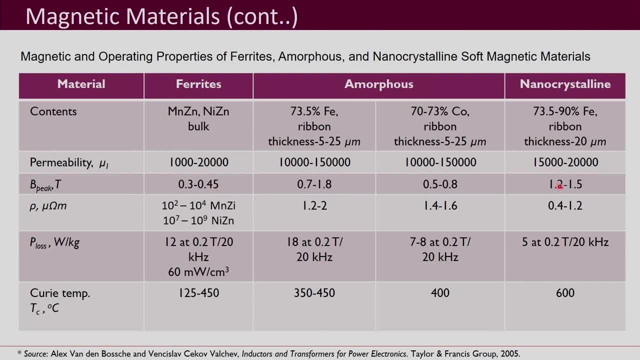 So you cannot use it for very high power applications, Whereas if you see here nano crystalline material, it can be used for relatively higher switching frequencies, I mean in the range of 100 kilohertz, And the flux density is also good. It is about 1.2 to 1.5, which is close to what we see for iron silicon material. 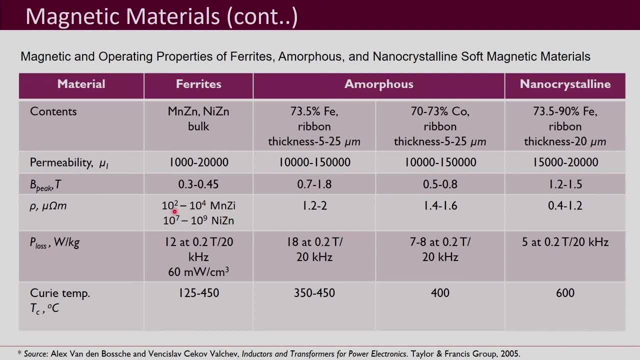 Then resistivity. if you see here ferrites have very good resistivity, very high resistivity, and these other materials have relatively have much smaller resistivities. Then p loss, The core loss, That is the p loss That is going to take place per unit. I mean this is watts per kg. in terms of that, the 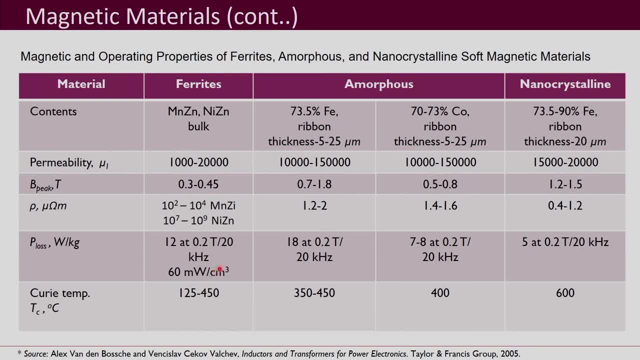 p loss data is given. So here you see, here, nano crystalline has relatively lesser your p loss as compared to others. Then curie temperature also. if you see, nano crystalline has got the highest curie temperature. So these are the important parameters that you should be looking for. 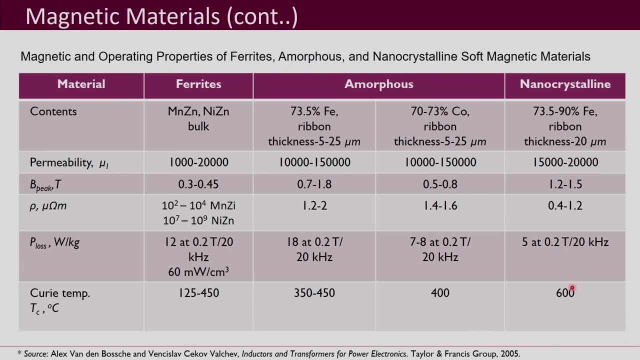 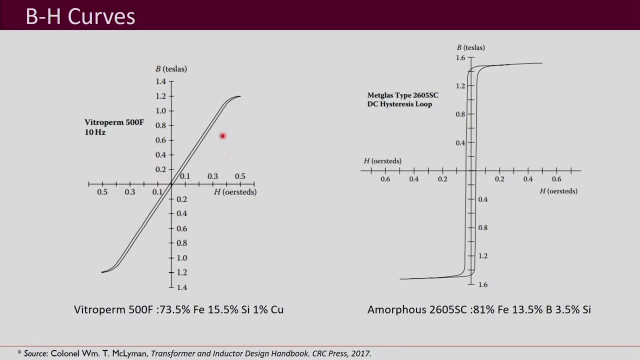 And then you can compare that which material is going to be more suitable for your design of inductors in transformers. Now, depending on the material, your b h curves can look to be very different. There are different manufacturers of magnetic materials and they make the magnetic materials. 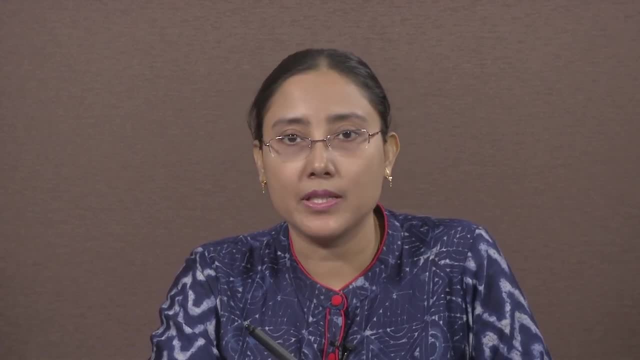 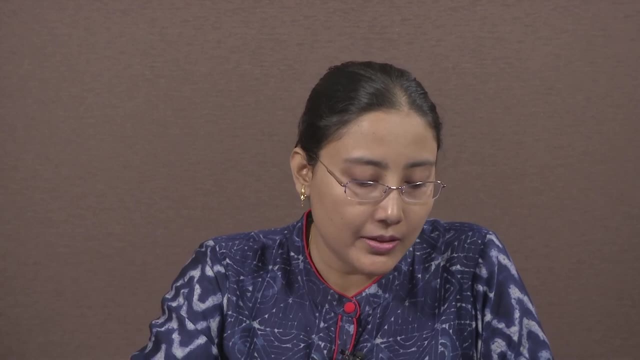 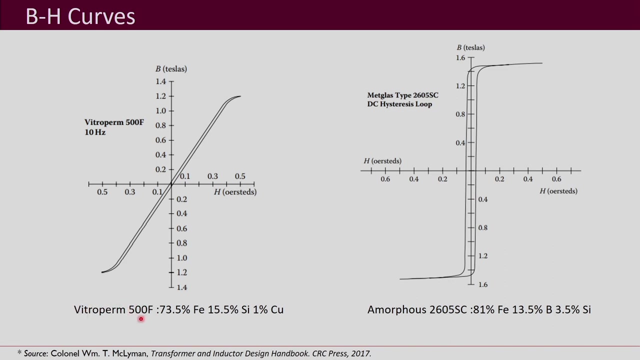 from different composition of different elements And, based on it, BH curve also, that is obtained is different. Now here this is this material: vitro perm 500F- this is the name of that material, and this has this composition: 73.5 percent iron, 15.5 percent silicon and 1 percent copper. 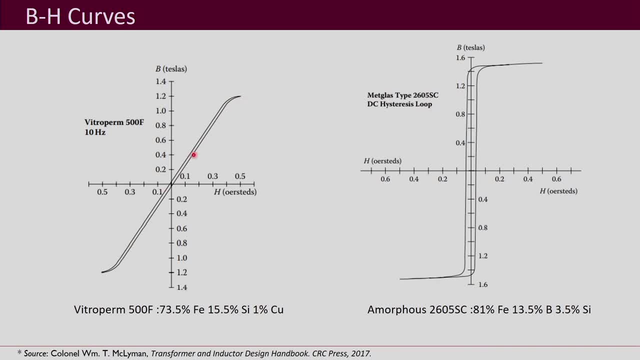 So the BH curve that you obtain is like this. And then here this is expressed in Ohrstedts: this is actually the CGS unit of your H magnetic field intensity, And then your amorphous 2605SE. this is another magnetic material. and here this BH curve is. 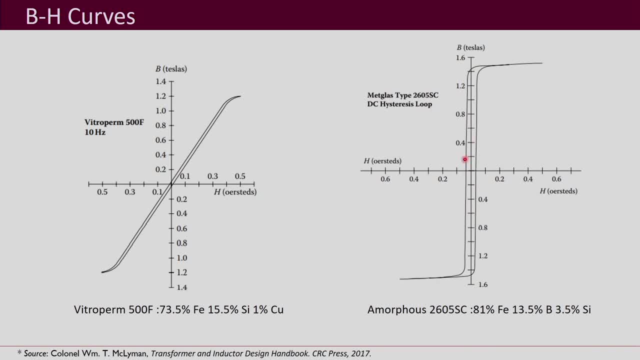 given, and you can see here that this BH curve is appears to be very different as compared to this one. Here your residual flux is much higher Flux density, although the coercivity is lesser, whereas in this case both the residual flux and coercivity are very small. 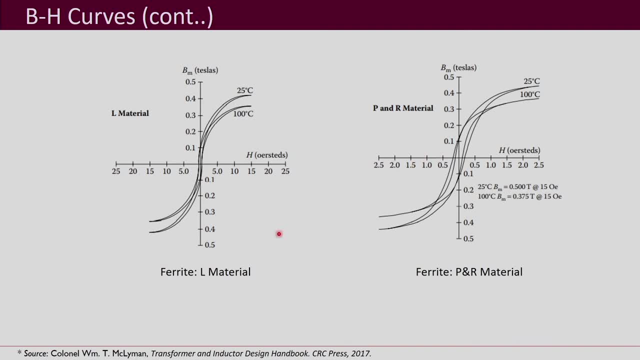 Then these are BH curves for your L material and P and R material. You can see that the BH curve shape is again very different. So here these are given for 2 temperatures: for 25 degree C and 100 degree C. So these are given for 2 temperatures: for 25 degree C and 100 degree C. So here these are given for 2 temperatures: for 25 degree C and 100 degree C. 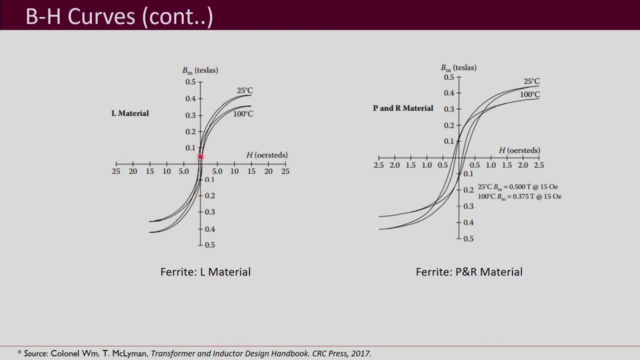 Now this is for L material. you can see that the BH curve is very thin, the width of it is very thin, whereas here you can see that that this for P and R material. they here, this BH curve is thicker, the width of it is higher. 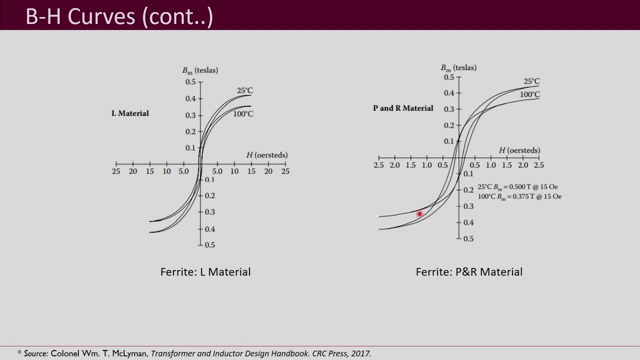 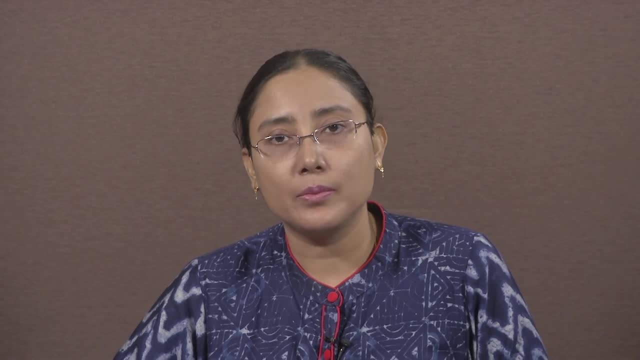 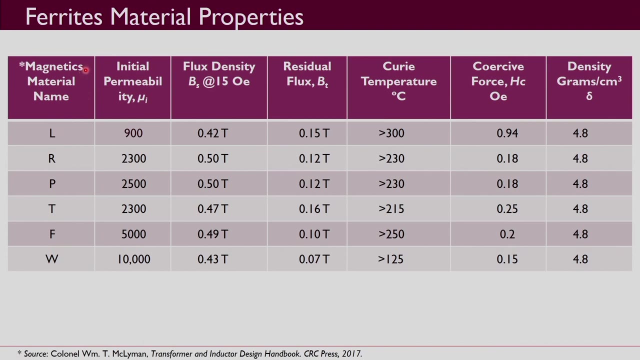 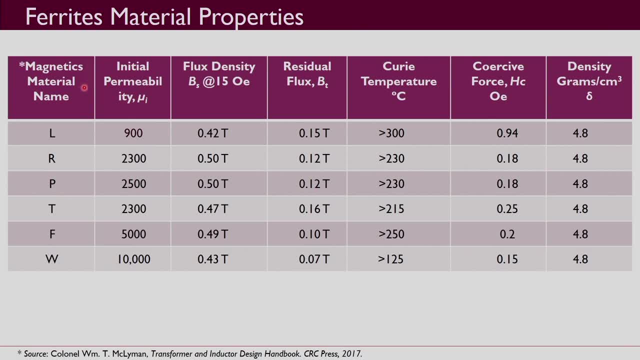 Now there is a manufacturer named Magnetics of your soft magnetic materials and they develop these ferrite materials and they have given different names to the different ferrite materials and these have slightly different compositions in them. So there are differences among them. So that is the data that is shown. so it is named as L, R, P, T, F and W. that is the notation. 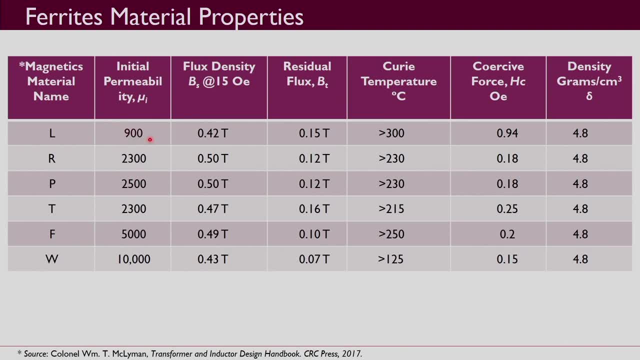 that is given to identify the material. So you can see here the permeability, so the best permeability is obtained for this ferrite material, W. and then the saturation flux density. it is more or less same but is relatively higher for your P and R materials and residual flux. you can see here that is lowest for this. 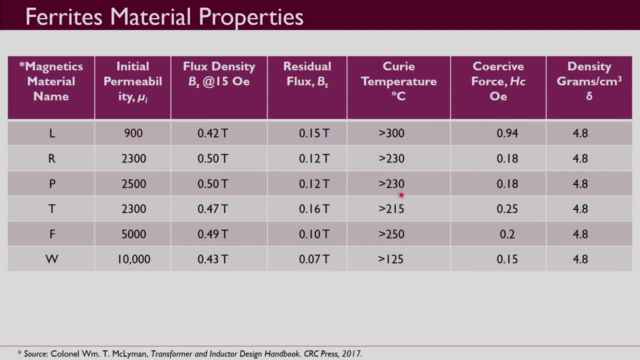 W. Curie temperature: again they also vary. this L material has got the highest Curie temperature. Then coercivity: again you can see here that lesser coercivity is for this W. So this is the material. So this is the material. 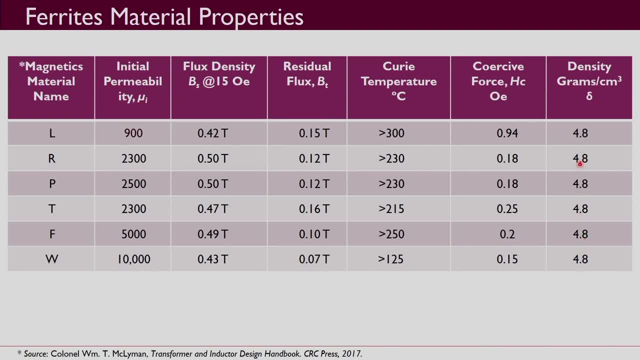 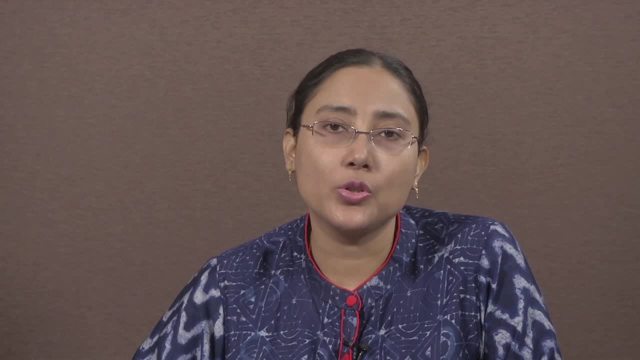 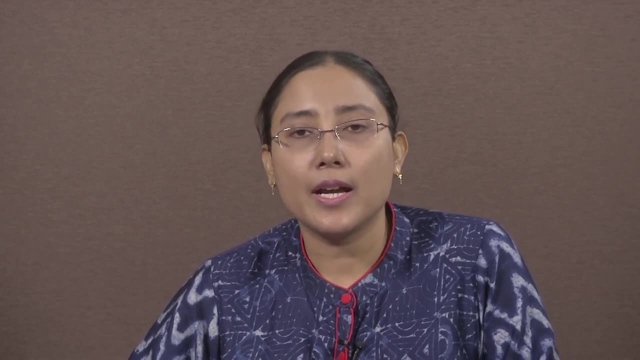 And the density is also provided, or density is the same for all of them. but density is also something you should be paying attention to, because if the density, it is the density which decides and how much volume you will be needing for a particular amount of weight. 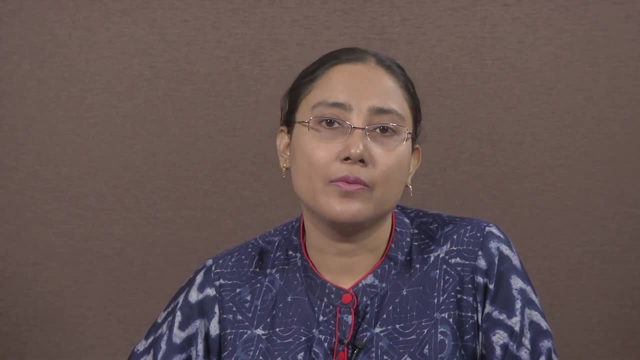 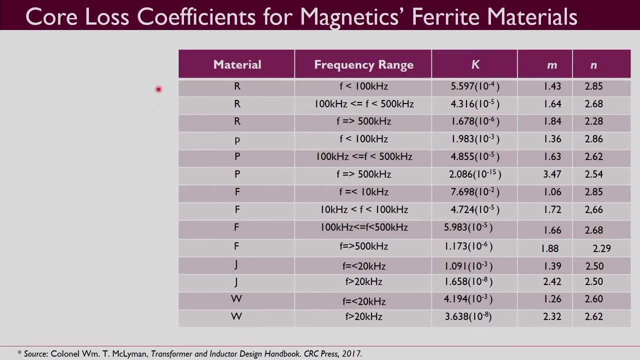 of that material. So we do not want very heavy and at the same time we do not want it the size to increase. Then when we discussed your core loss calculations at that time I told you that these coefficients are important. So you may recall that your this core loss per unit volume was given as your K f power. 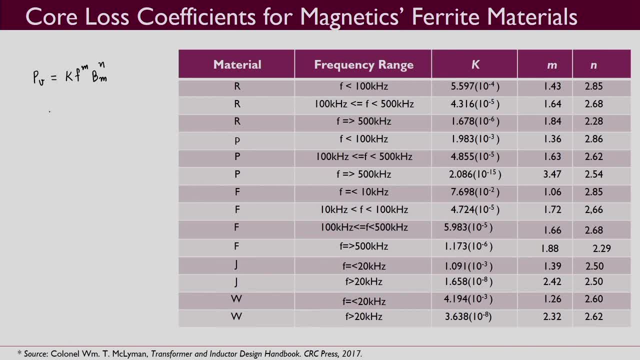 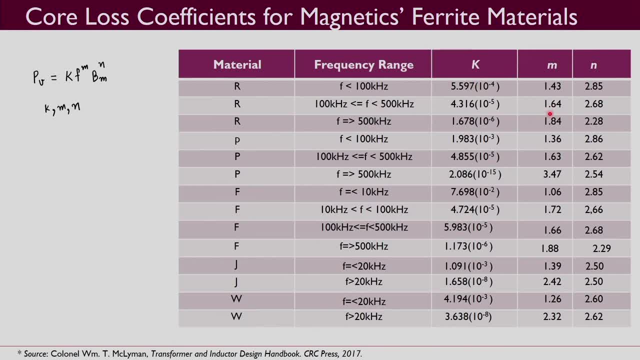 your core loss. So those data are provided by the manufacturer of the materials. You can see here this is for the same ferrite materials which are manufactured by your magnetics, So their frequency range is given. So their frequency range is given. 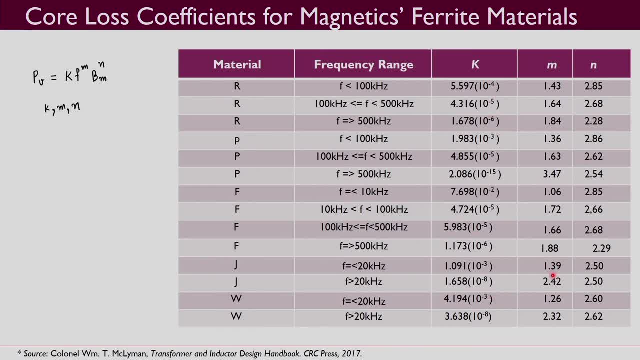 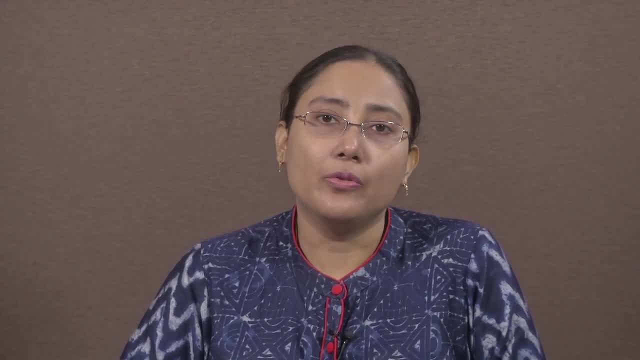 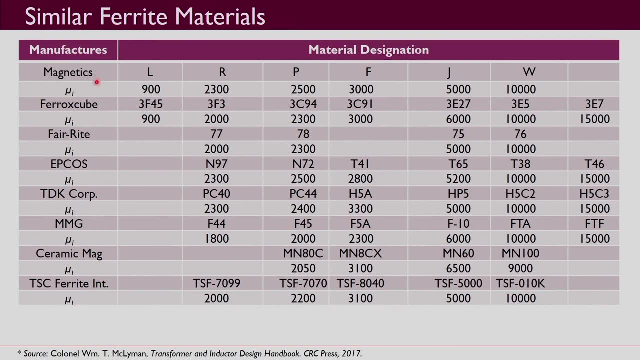 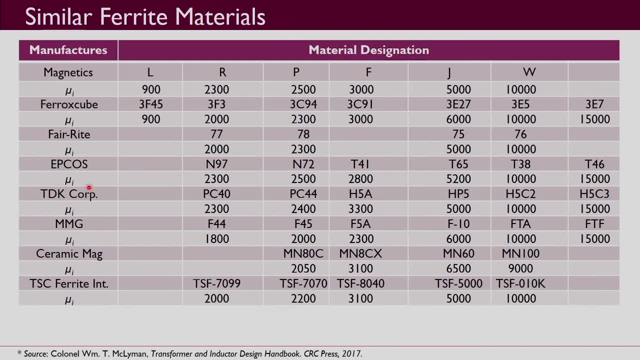 here it is listed, your Magnetics Ferrox, cube, Ferri, Epp, Cos, TDK and so forth, and they all make different, different magnetic materials. but there are some similarities in the other materials, similarities among them. I mean, you can categorize them as which are the similar magnetic materials? 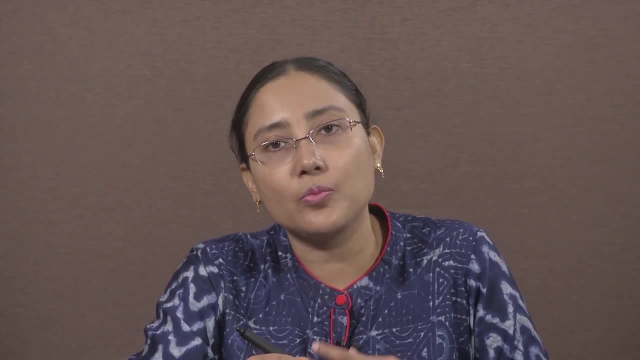 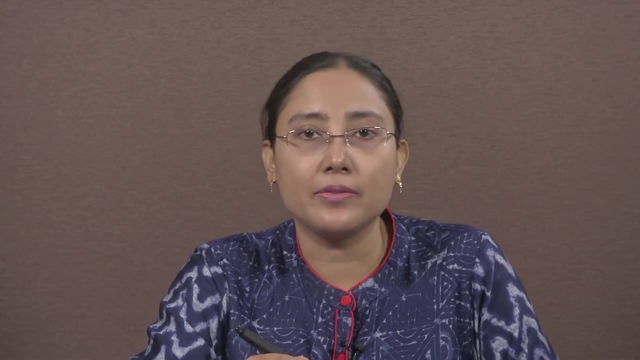 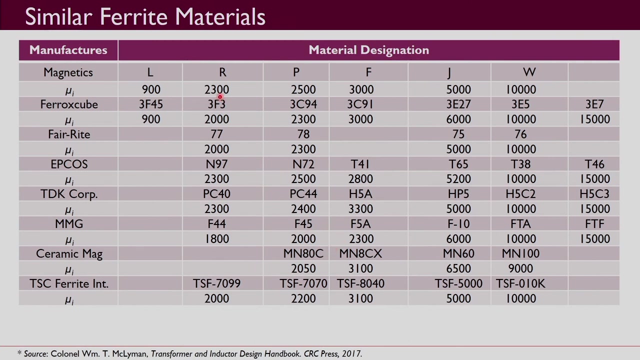 So that is easy for you to choose, that if suppose you are not able to get the magnetic material of one manufacturer, similar magnetic material from other manufacturer you can obtain. So that is what this table is showing, but note that the material may be similar but 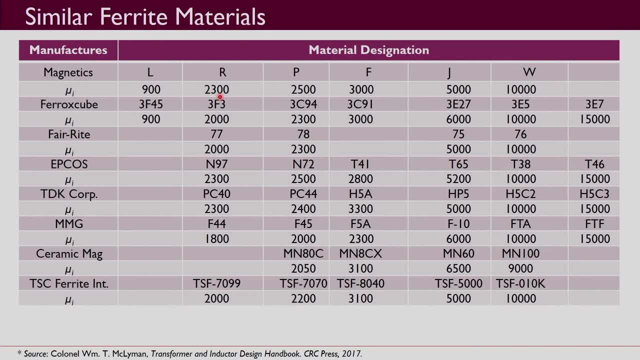 their part numbers or their designation, the way in which they are denoted are different or identified are different. Now here you can see this is by magnetics. magnetics- ferrite materials are denoted like this: LRPFJW and so forth, and this by ferox cube. they like to give this number 3 before.